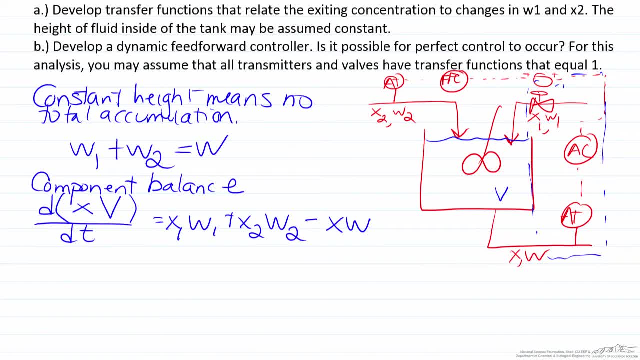 We'll assume here that V is a constant, so therefore we'll have V dx dt equals X1 W1 plus X2 W2, minus X times X2 W2.. Okay, So that's the combination of the two streams: W1 plus W2.. 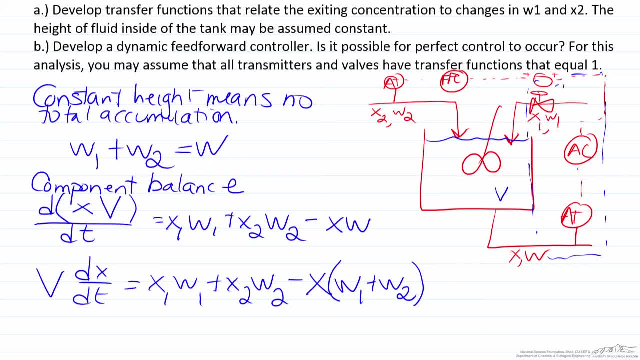 So the important point to note here is what variables are allowed to deviate. so therefore, obviously X can deviate and the problem statement says that X2 can deviate and the valve is being adjusted. so therefore we know that W1 can also be adjusted. 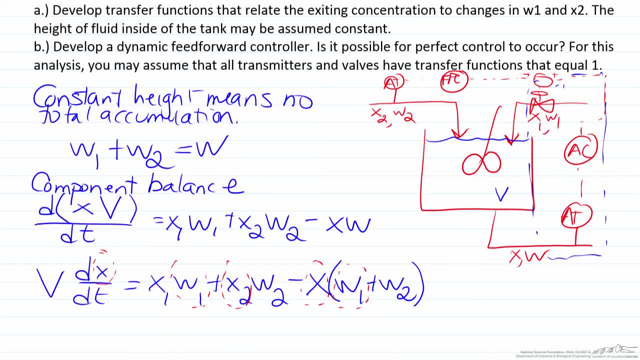 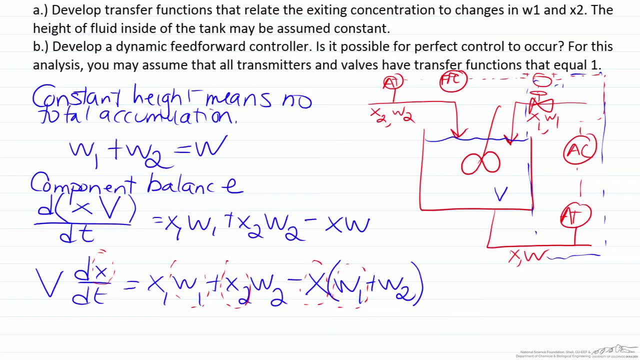 So what we note here is that we have a good number of variables present here, so we now have to, We put this into deviation variables, and we also have the last term which needs to be linearized. So to do all of this, we're going to use an equation which has been developed and actually 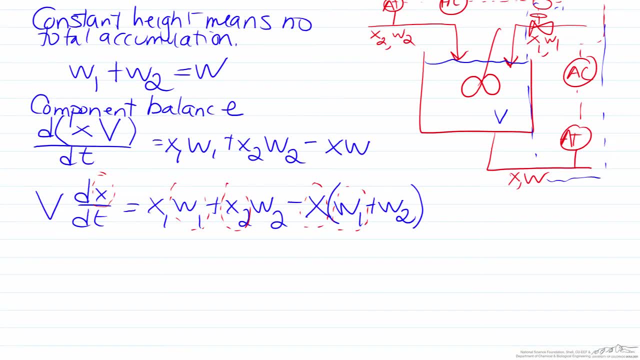 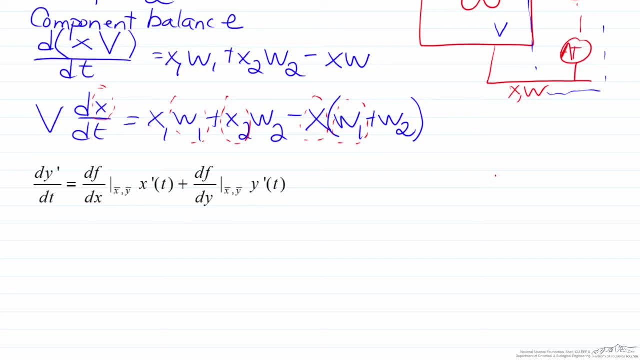 has been derived in a previous screencast in order for us to handle this equation. So in this case here we'll actually have a third variable here, because we have W1,, X2, and X, but the logic here follows. therefore, what this leaves us with is V, dx, prime, dt equals. 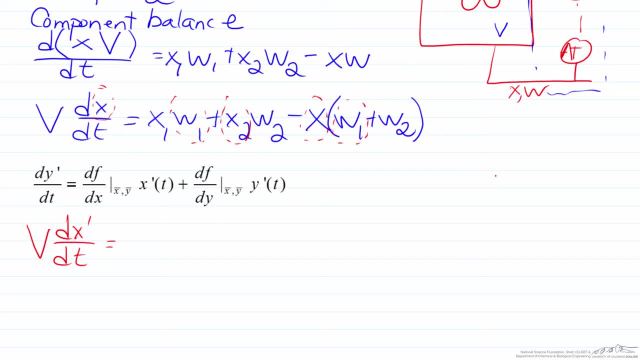 the derivative with respect to a variable. here we'll start with W1, so we take the derivative with respect to W1, we'll have X1 minus X, and again these will be evaluated at the bars multiplied by W1 prime plus the derivative. we'll do X this time, so X. 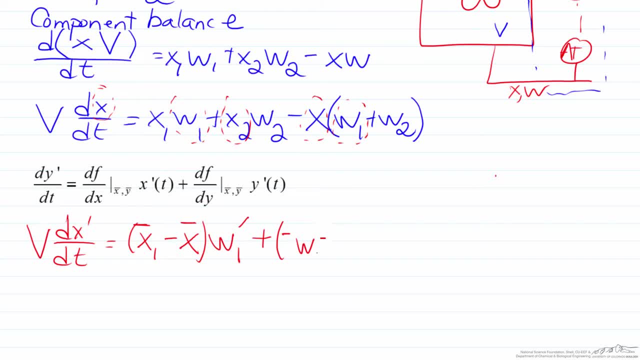 is only in one place. so the derivative here will be negative, W1 minus W2, and these will be evaluated at the bar values, So W1, multiplied by X prime. And then we'll take a look at our third variable here, which is just W2 bar the derivative. 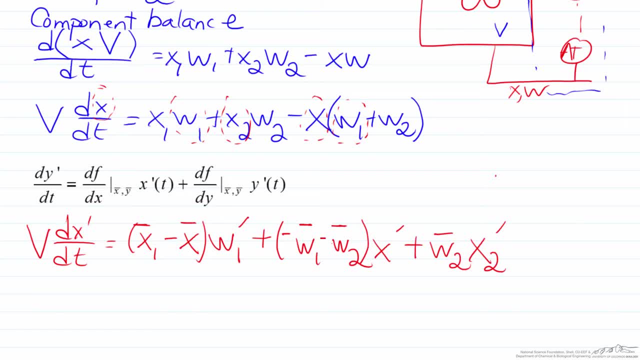 of the second term multiplied by X2 prime. And a point to note here is that, technically, since W2 in this analysis and X1 in this analysis are assumed to be constant, the bars are not absolutely necessary here, but just for simplicity's. 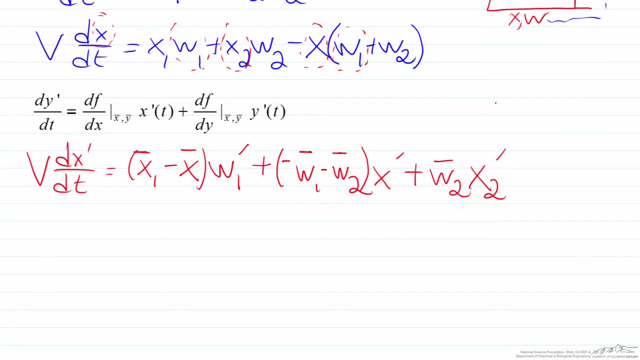 sake, we will keep them here. Now we'll take the Laplace transform of this. so therefore, the only thing of real interest here to take the Laplace transform of is the value on the left hand side Again, since we're in deviation variables, the f. 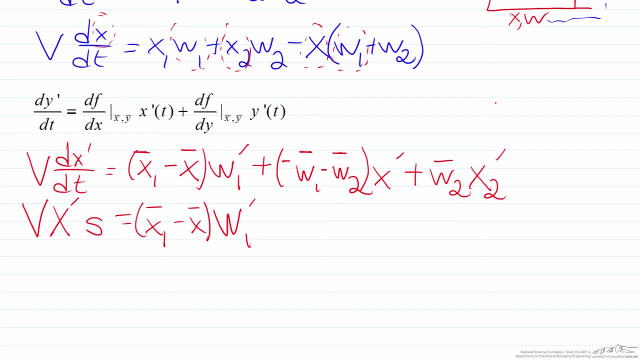 of 0 term goes to 0, so we're just left with: on the left hand side, the derivative term becomes v, the coefficient times, x, prime s and the other terms. since they're just variables, the Laplace transform is the variable, except in the Laplace domain. We can now move. 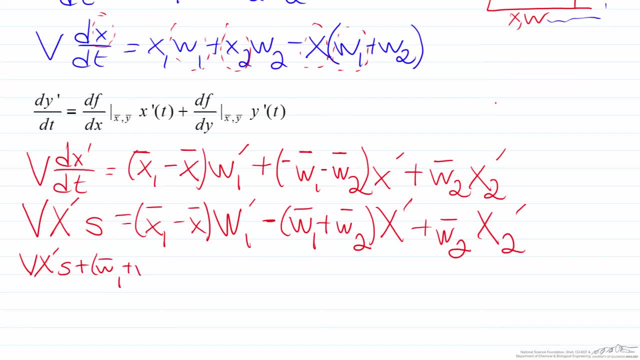 the x prime term over Again. this will now become a plus and we'll have two separate transfer functions here, one representing how a change in x2 affects a change in x and one showing how a change in w1 affects it. So we'll divide everything now by w1 bar. 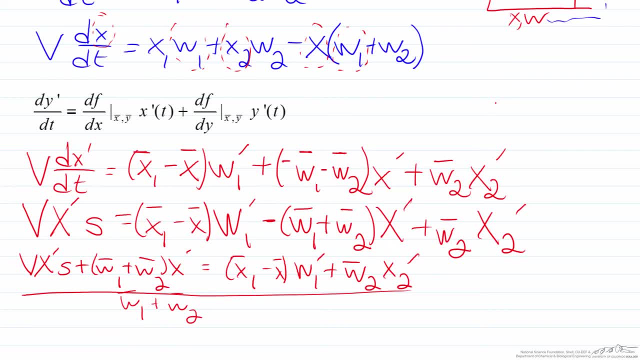 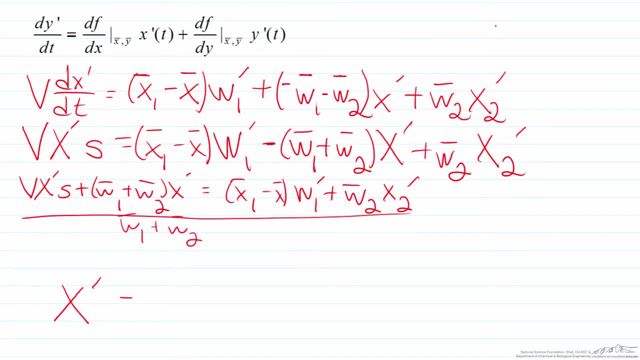 plus w2 bar to get everything into tau s, plus 1 form to get into standard form. So what this leaves us with is that x prime is going to equal x1 bar minus x bar divided by w1 bar plus w2 bar. 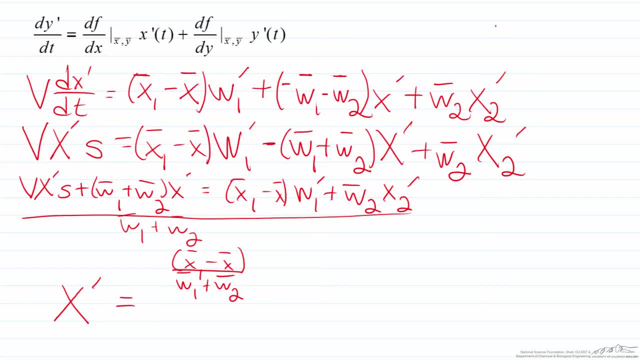 So that will be the difference between the two terms. To be representative of the gain, we'll divide that by v over w1 bar plus w2 bar, s plus 1, and this will be w1 prime plus w2 bar over w1 bar plus w2 bar, divided by the same denominator. 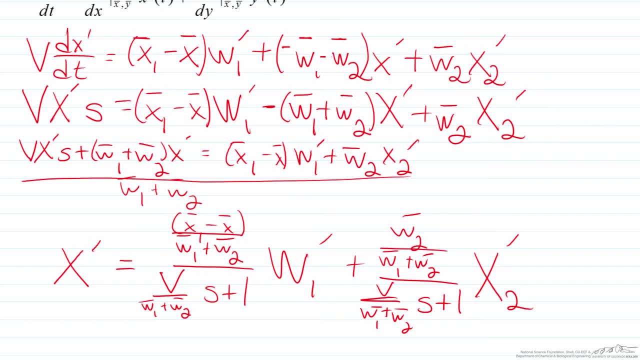 as we had before. Could we represent w1 bar plus w2 bar as the steady state total flow rate? Yes, we could, but here we'll just keep it as a note. What we'll now do for simplicity sake is we will recast the two terms in the numerator for w1 and x2, we'll 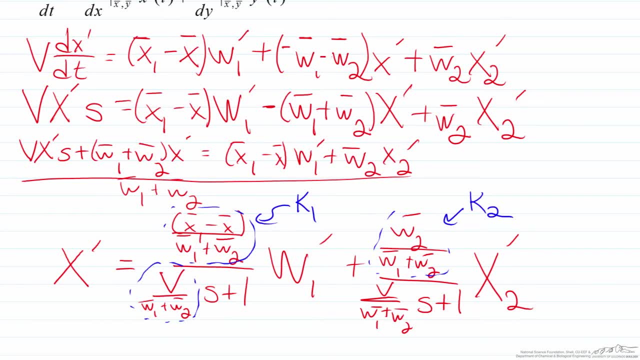 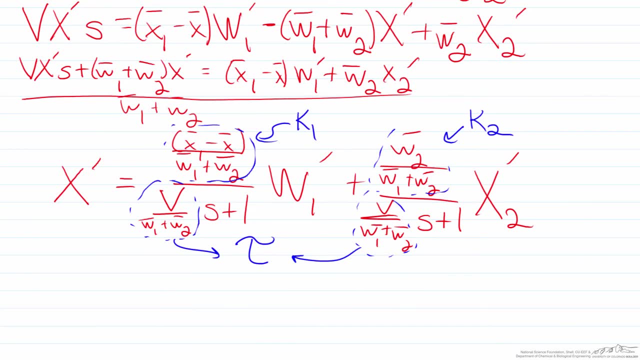 recast as the gains k1 and k2, and both denominators have the same time constants, so therefore that would just be tau. So part was asking us to develop a dynamic feed forward controller and to determine if perfect control was possible, and it was given that all transfer functions. 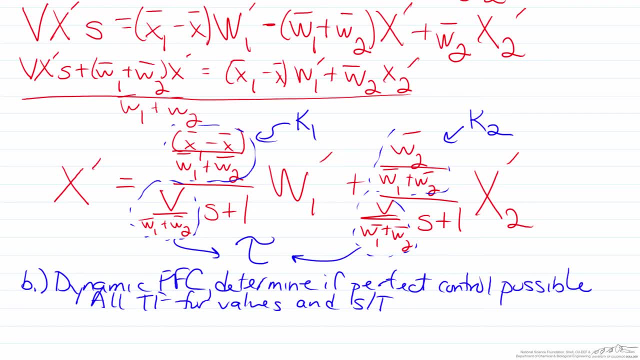 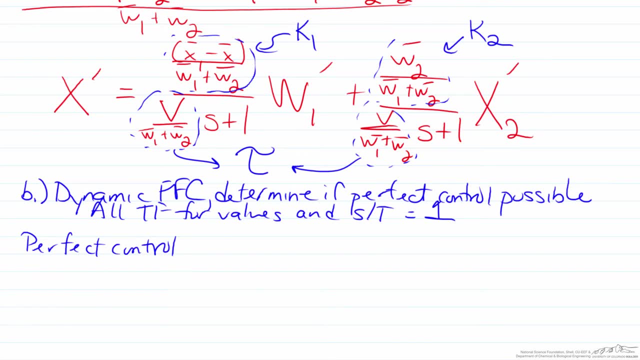 for valves and sensor transmitters equal to the same time. so that is thou That's equal to one. So, in order to get perfect control, remember that what perfect control represents is a disturbance has no influence on the controlled variable, So you can assess perfect control. 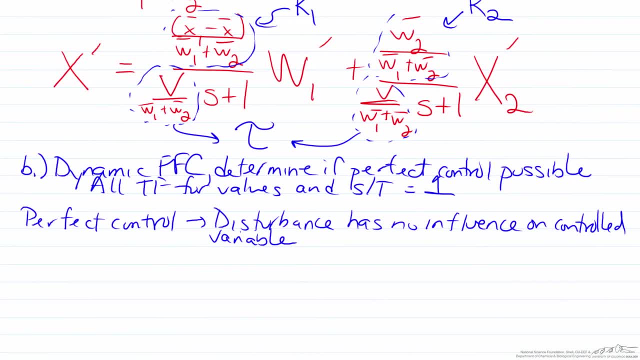 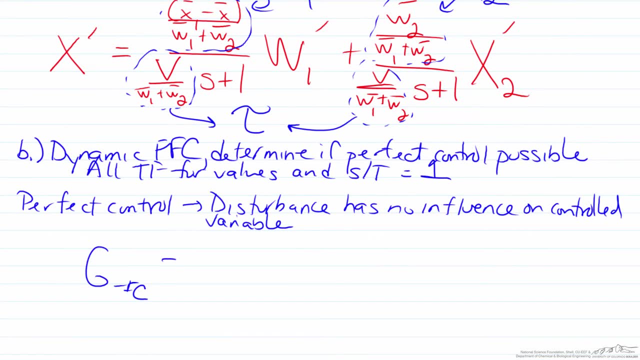 using block diagram analysis, which has been done in a separate screencast. we're not going to discuss that here, but what we know is that the transfer function for perfect control for a feedforward controller can be defined as negative gd over gt, gv, gp. So gd represents. 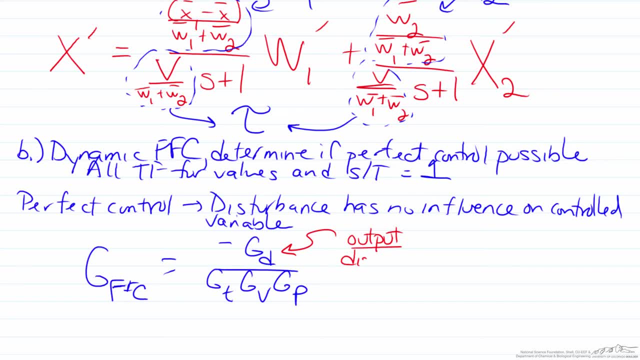 how the output variable is influenced by a change in the disturbance variable. gt is the transfer function for the sensor transmitter of the disturbance variable, gv is the transfer function for the valve and gp is the process transfer function for the relationship between between the output variable and the manipulated variable. So if we try to match these with, 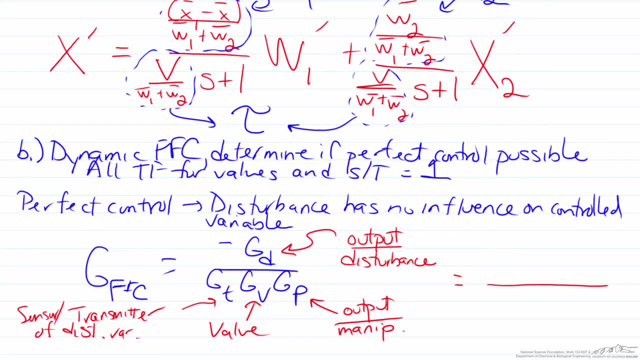 what we've seen so far is gt and gv. in the problem statement are explicitly stated that they're equal to 1.. If I look at the equation I've just developed, I've found the transfer function that relates how the output, which is in this case x, the exiting concentration. 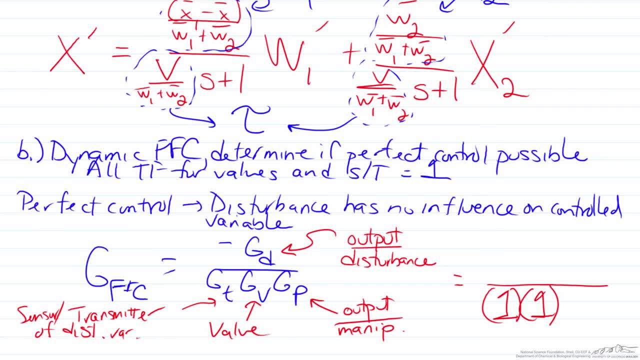 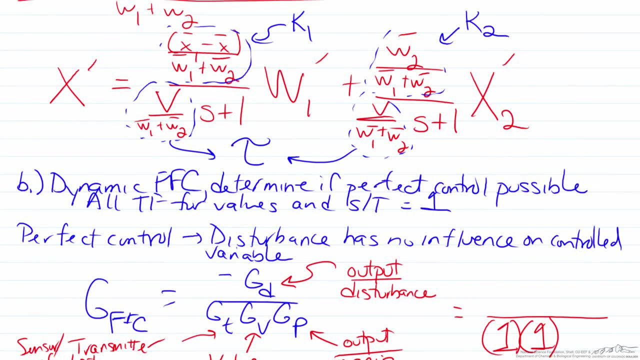 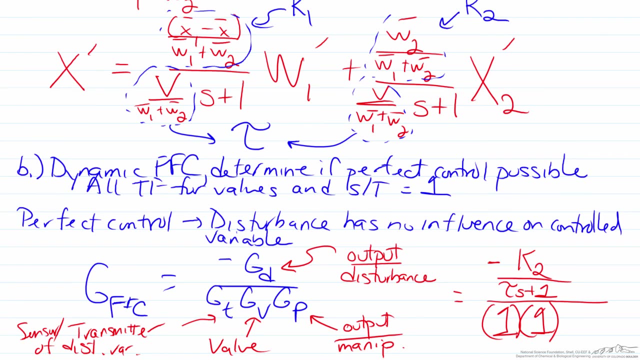 is influenced by a disturbance. In this case the disturbance is the concentration of the wild stream. So if we see how that we recast these, we'll show that this transfer function is just negative k2 over tau s plus 1.. And similarly how the manipulated variable in 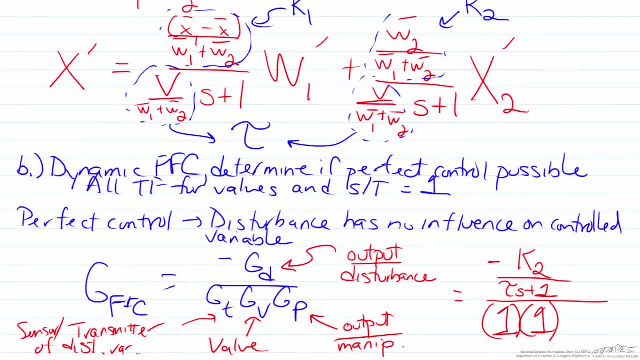 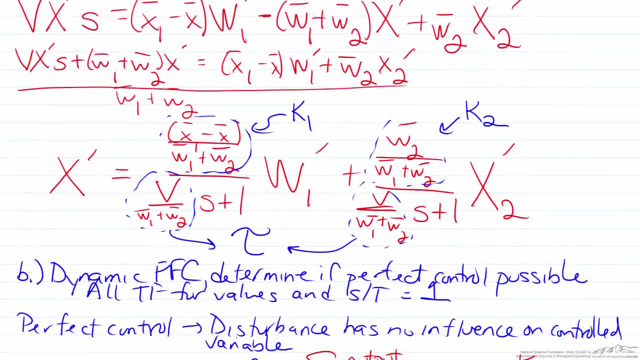 our case the manipulated variable is the one with the valve on it and we call that represented the stream w1, as you can see in the diagram here. So therefore, that transfer function we also obtained from doing the mass balance, and this will just be k1 over tau s plus 1.. 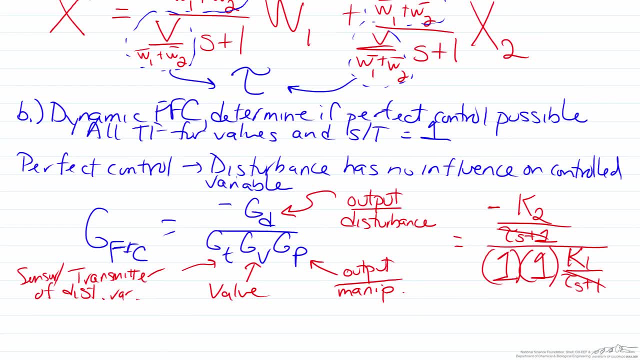 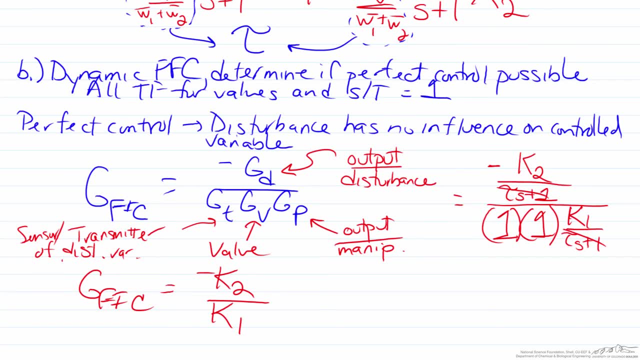 So in our case here the tau s plus 1's cancel and we're left with a feed forward controller which is just a gain. here it's a zeroth order transfer function of negative k2 over k1.. So, based on our analysis, since k2 and k1 are both positive values, what this means is that here perfect. 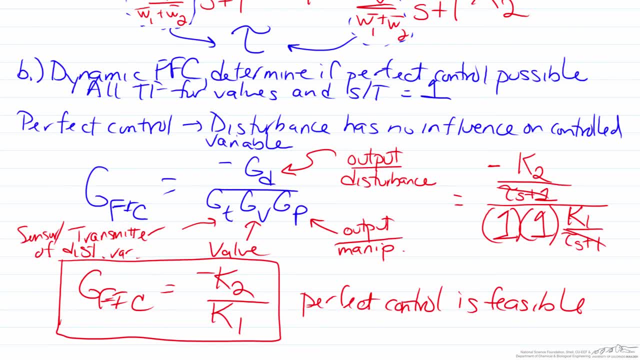 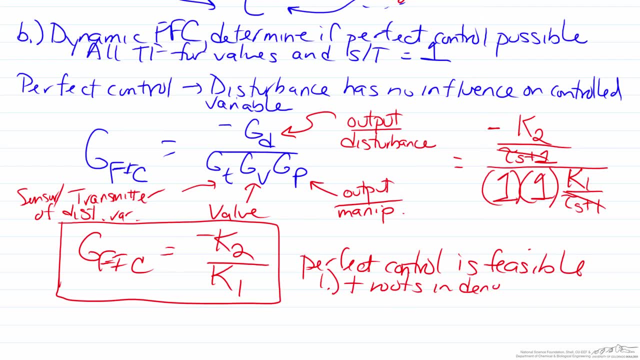 control is feasible. Why? Because this transfer function is feasible, and the two major issues here that we would want to check on are positive roots in the denominator. those are bad. we don't have an issue with that here, because there are no powers of s. and the second is: 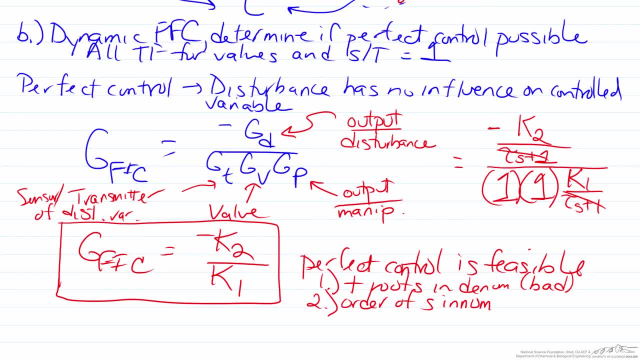 that the order of s in the numerator must be less than or equal to the order of s in the denominator, and in this case the order is both zero. So therefore, this feed forward control is perfectly valid and perfect control is possible, assuming that we had perfect models.